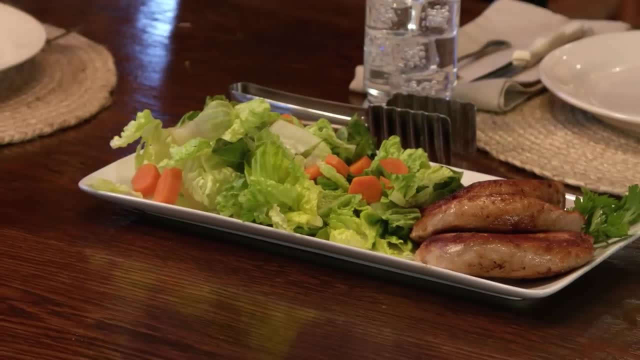 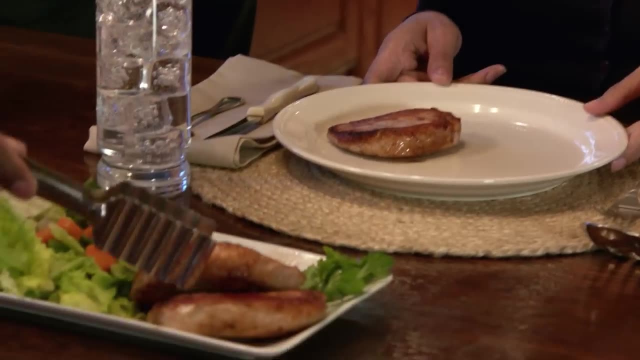 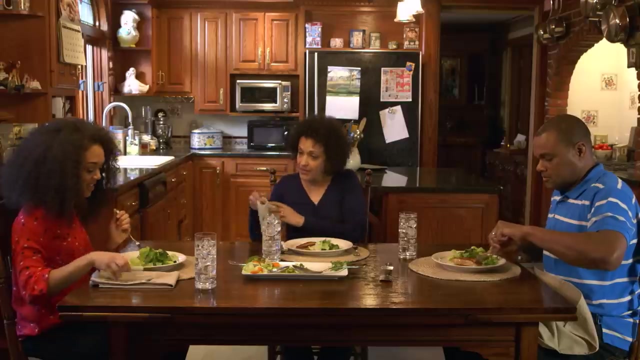 We all know how well meat and vegetables go together in a meal. But before he cooked for his family, Terrance had to be careful to keep his lettuce and pork chops separate. Why? Because harmful bacteria from the raw meat can cross-contaminate other foods and may make those eating it very sick. 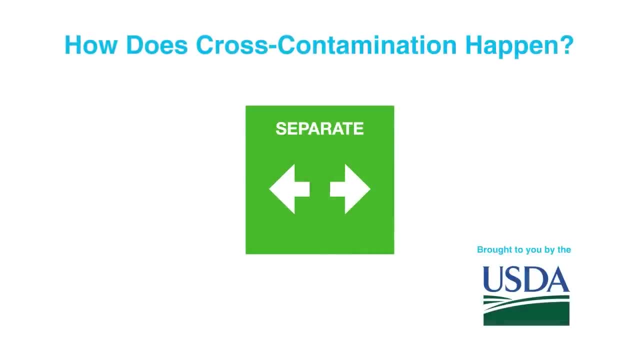 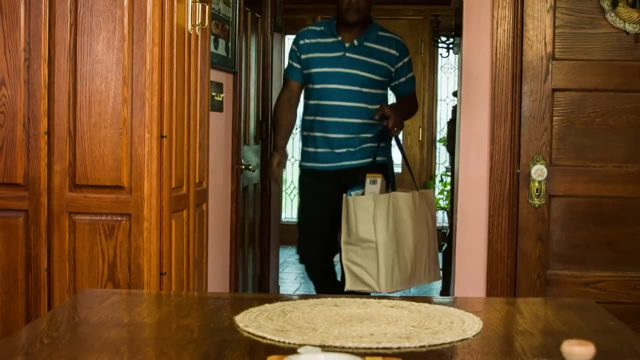 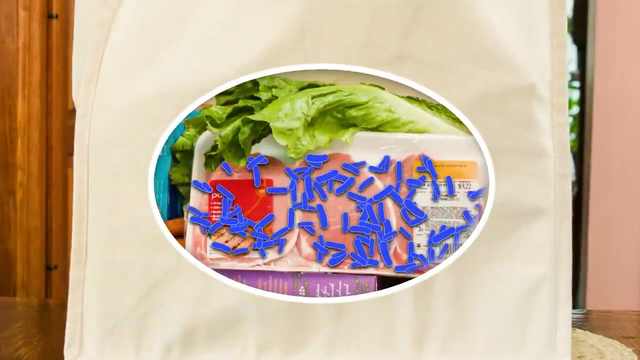 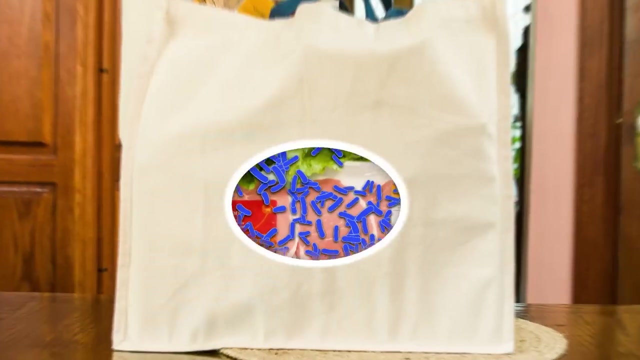 If Terrance had forgotten to bring separate bags for his meat and produce at the grocery store, any bacteria from the pork chops could have cross-contaminated the head of lettuce. These bacteria can come from the juices of raw meat or even just the products or product packaging touching when no visible juices are present. 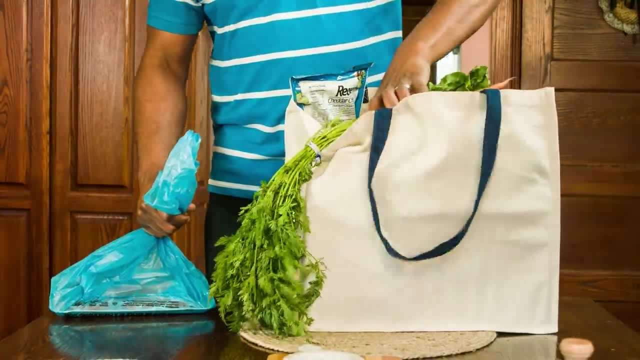 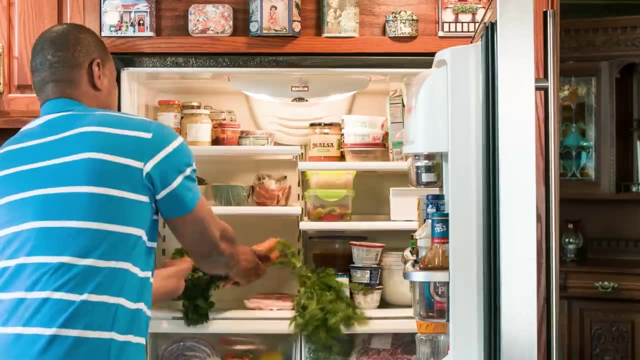 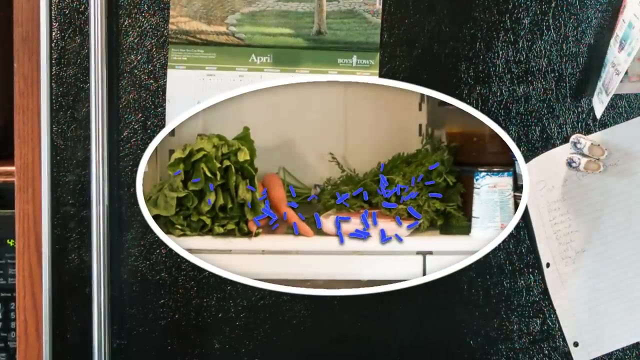 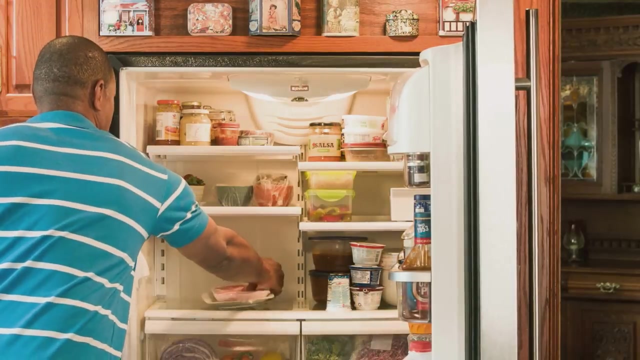 Fortunately, Terrance kept his meat separate. He kept his raw meat and produce separated, But his food isn't out of danger yet. Cross-contamination can also happen in his refrigerator. But Terrance remembered to keep his raw meat and vegetables separate. 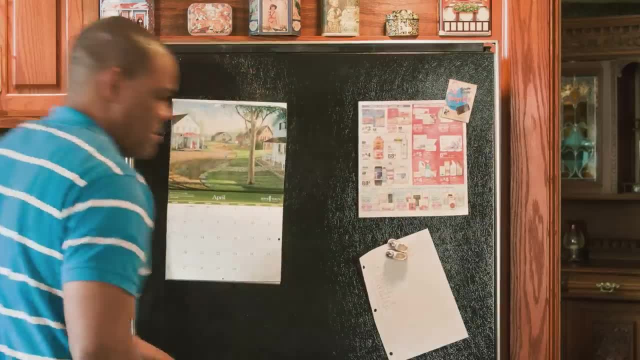 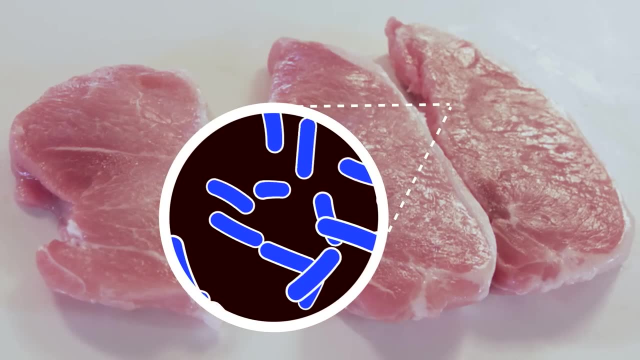 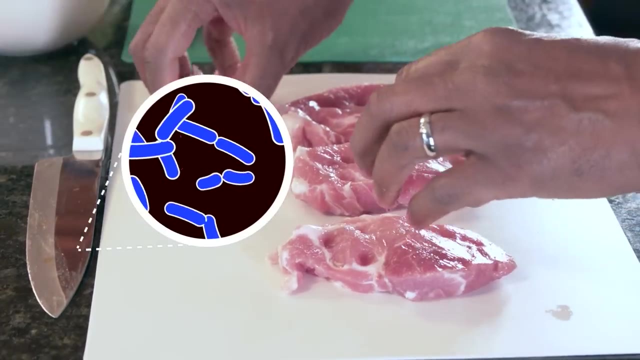 More cross-contamination avoided. Terrance must be very careful when cutting his meat because, though he can't see it, there could be bacteria on this pork. He can spread this bacteria from the meat to his utensils, his vegetables and his kitchen towel. 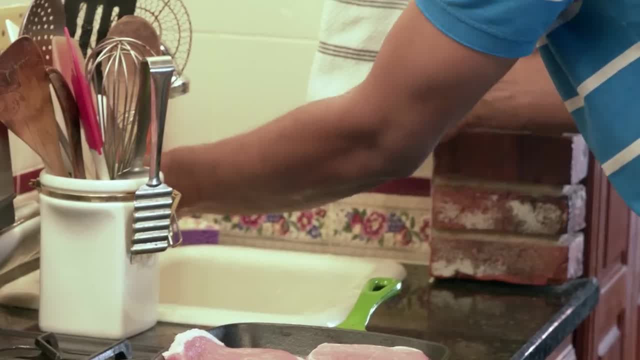 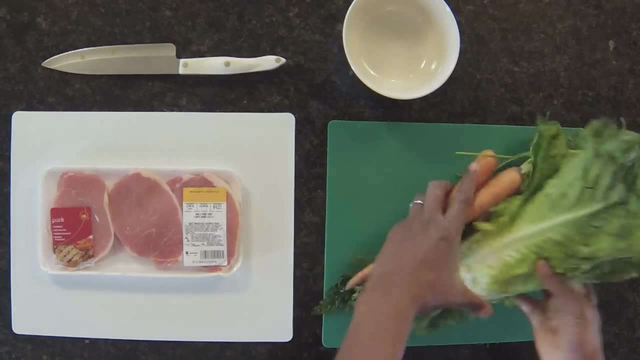 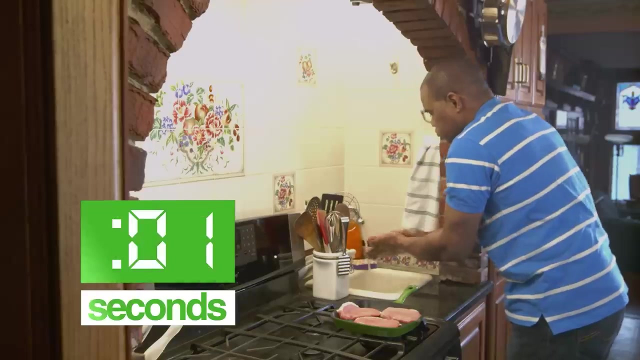 If he does not wash his hands well after touching the meat, cross-contamination is far more likely. But fortunately for his family, Terrance was careful. Terrance washes his hands with soap and warm water for 20 seconds after handling the pork. 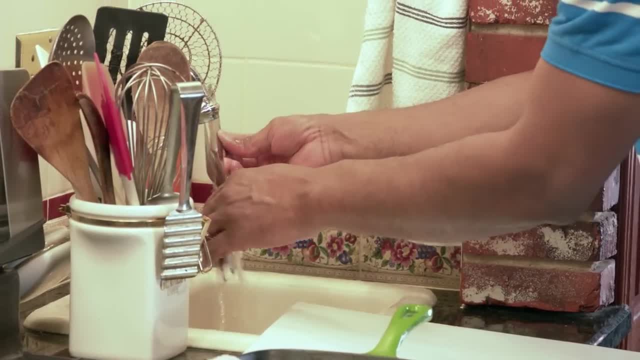 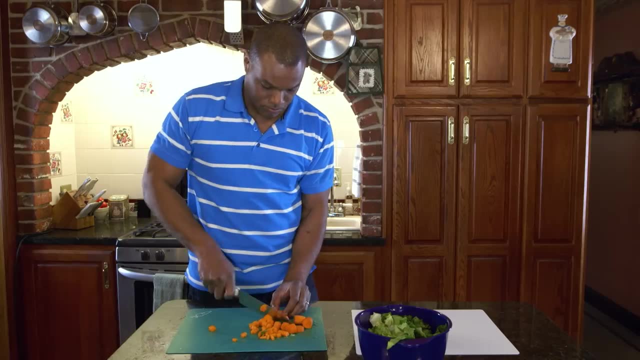 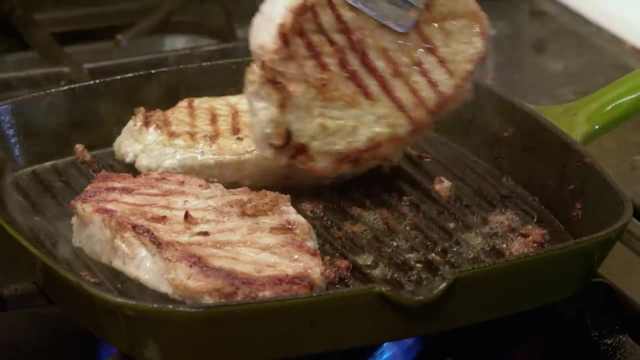 He also washes the cutting board and utensils. He keeps his vegetables separate from his raw meat And he's careful to keep the cutting board and utensils used for the meat away from his raw vegetables. All Terrance has to do now is use a food thermometer to be sure that his meat is safely cooked. 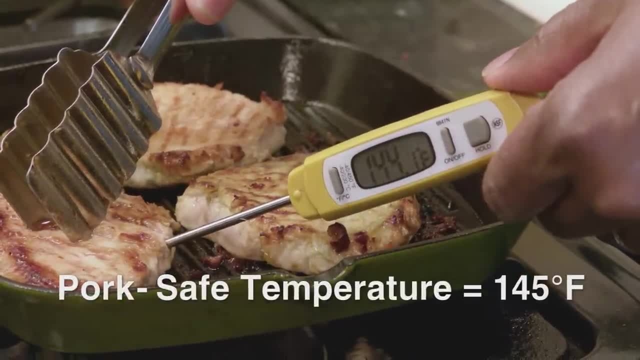 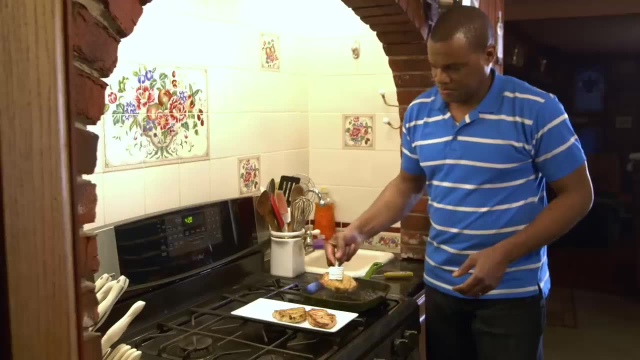 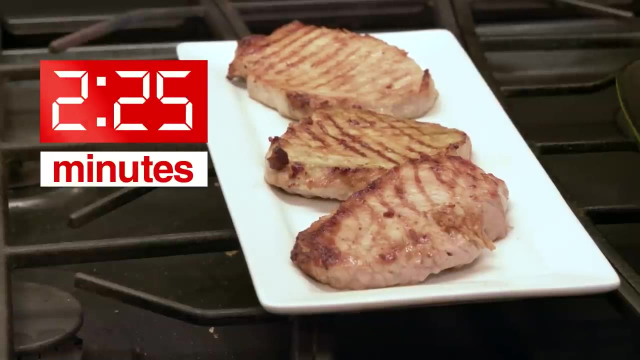 The pork's internal temperature is safe at 1°C. All whole cuts of pork, beef and lamb require a three-minute rest time before they're safe to eat. During these three minutes, after meat is removed from the heat source, its temperature remains constant or continues to rise.